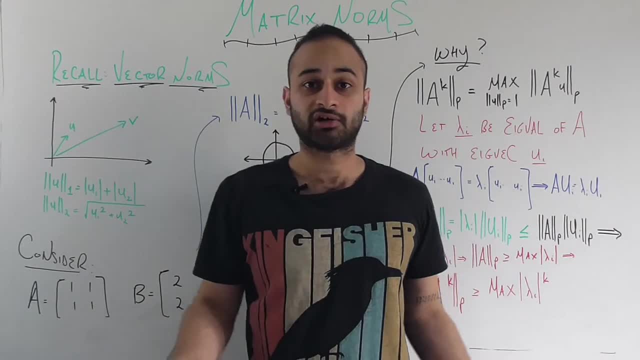 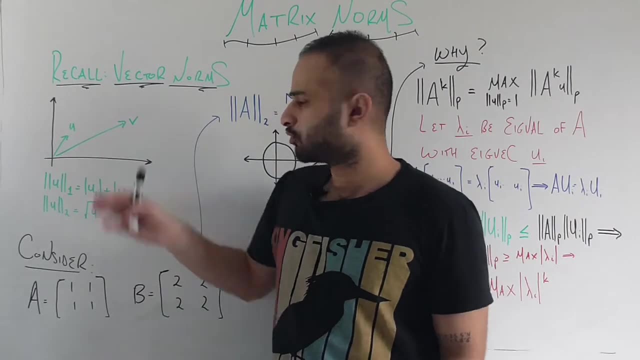 this graph with vector v and vector u and I asked you which vector is, quote-unquote, bigger? I think most people would say vector v, because it just looks longer. maybe maybe it just looks like it's more intense in magnitude. but without some mathematical foundation it's hard for us to tell. 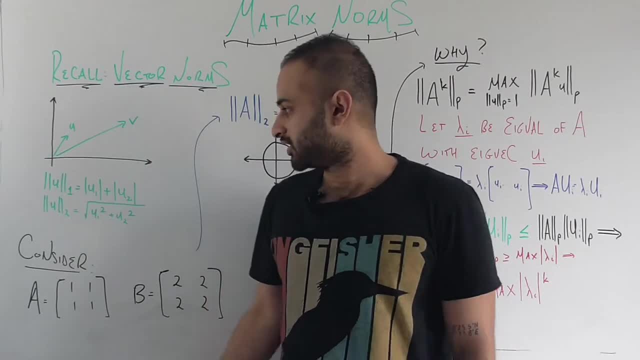 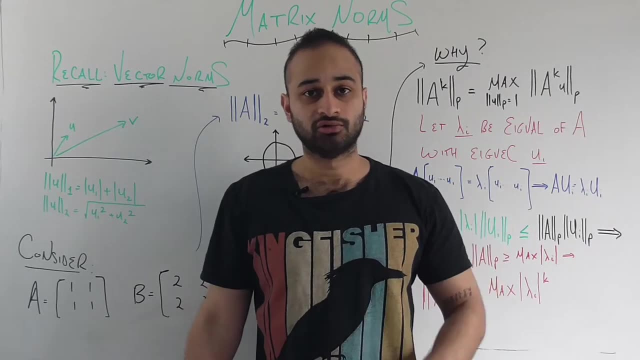 objectively, and that's why vector norms were created. For example, we know the L1 and L2 norm as probably the most popular. The L1 norm, remember, is just the sum of the absolute values of all the components and the L2 norm is the square root of the sum of the squares of all the components. and 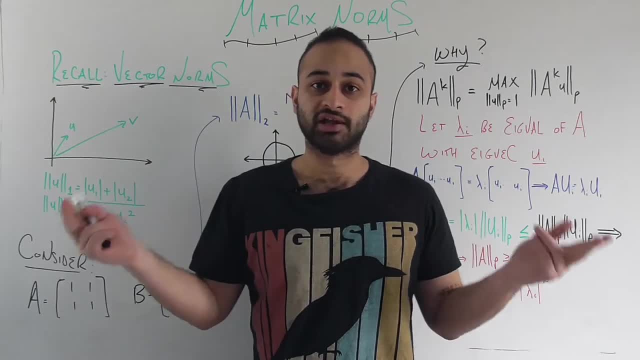 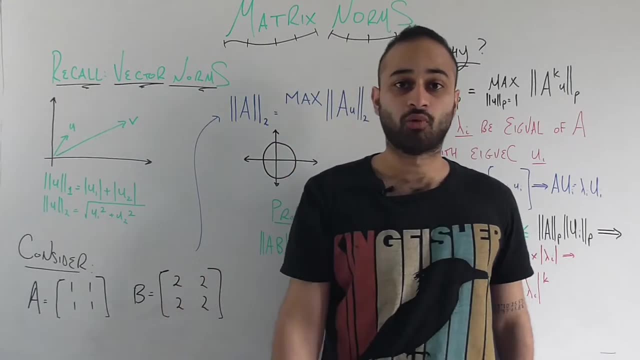 either way, we're going to find that v is bigger than u. Now you can imagine we want to do a very similar thing with matrices, If I give you matrix A, which is just full of ones, and I give you matrix B, which is just full of. 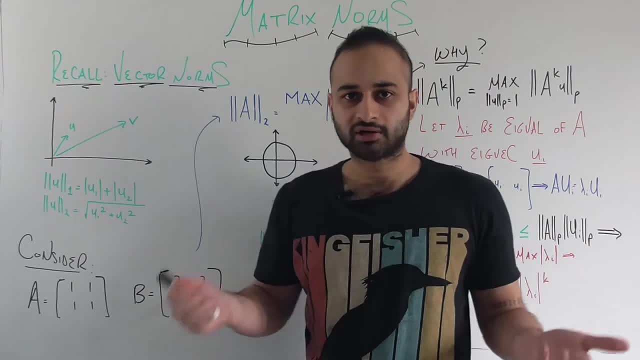 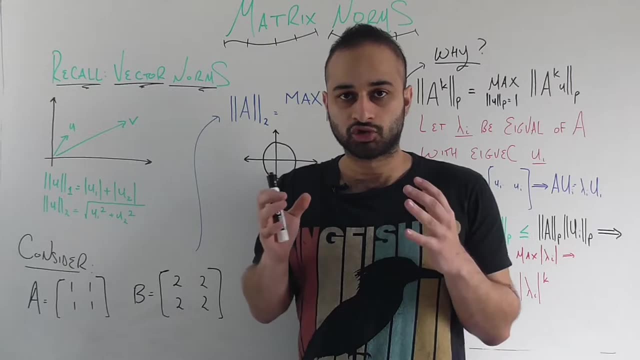 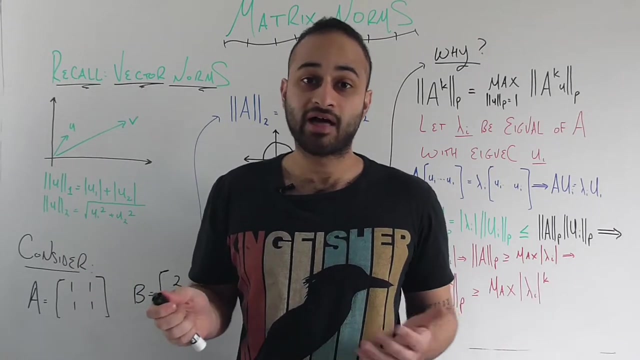 twos, then most people would say that B is bigger than A because it seems to just contain bigger numbers and every number is double that of A. but how do we make this notion concrete? And that's where the matrix norm comes in. The very clever thing people did is that there's no new math with 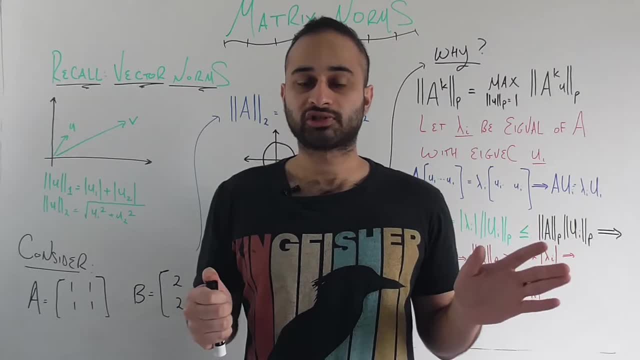 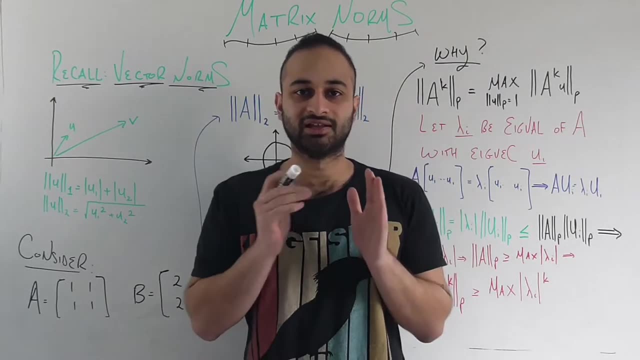 matrix norms, because we're going to base all of it on vector norms. How do we do that? We go back to the definition of a matrix, Not that it's just some kind of grid of numbers, but rather that it's a linear transformation. 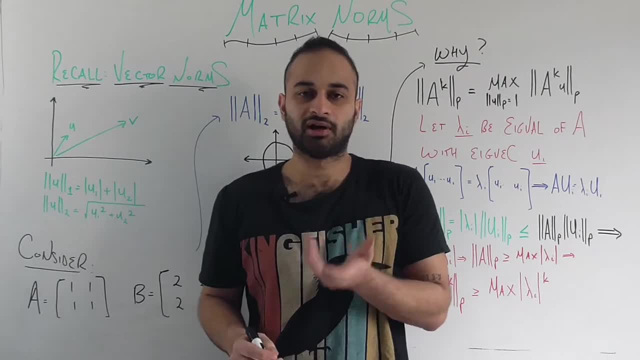 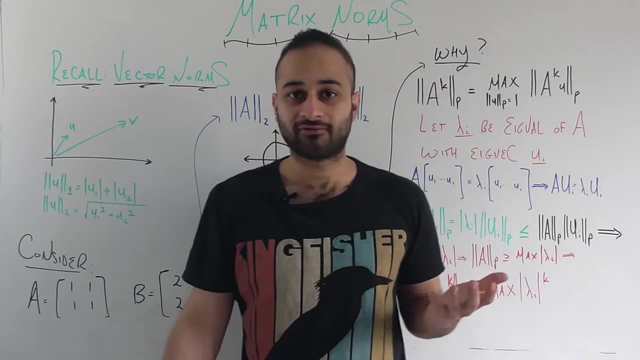 Another way to say that is that it's a function that takes some vector and maps it to some other vector. That other vector might be in the same space as the input if it's a square matrix like these guys, but it doesn't have to be. If it's a rectangular matrix, then it could take some vector. 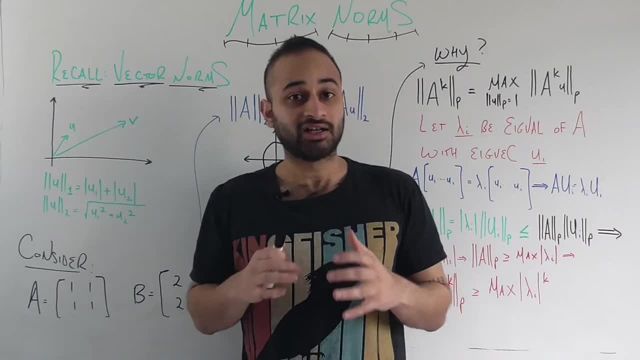 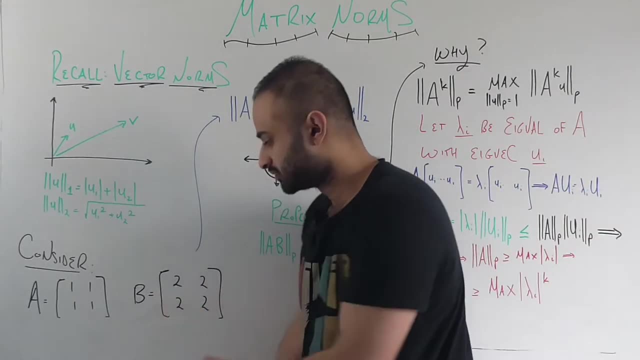 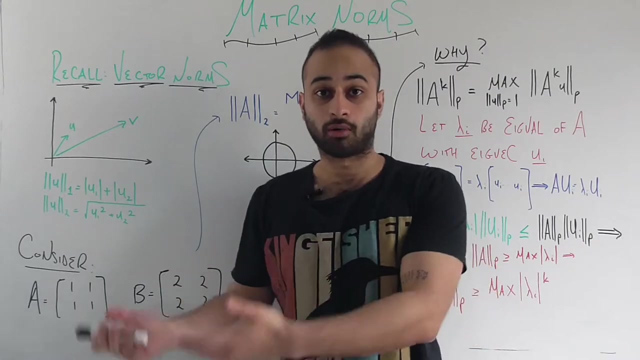 map it to a different space. But either way, we're going to be defining a matrix norm in terms of how big that output vector can get. For example, you can imagine that this B is going to be able to map input vectors to bigger output vectors, and by bigger I mean vectors with bigger norms. So how? 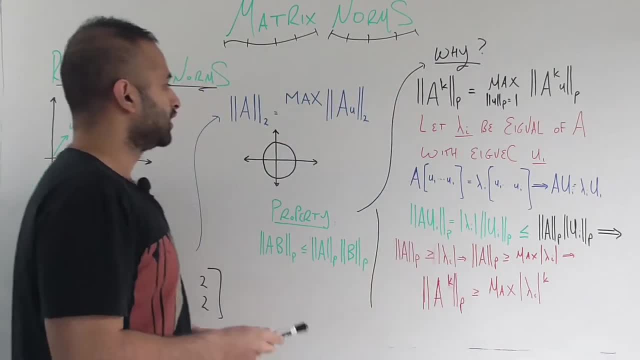 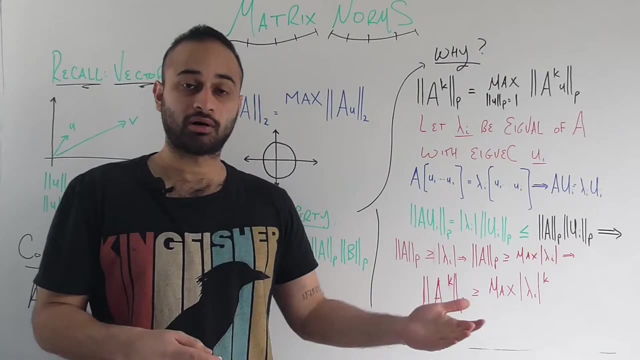 do we make that mathematically concrete? Let's go ahead and take a look at the definition. So we're saying that the L2 norm of a matrix and again, just as with vector norms, you have to specify the number in terms of which norm you're taking. Are you taking a 1 or 2, whatever norm? So just to 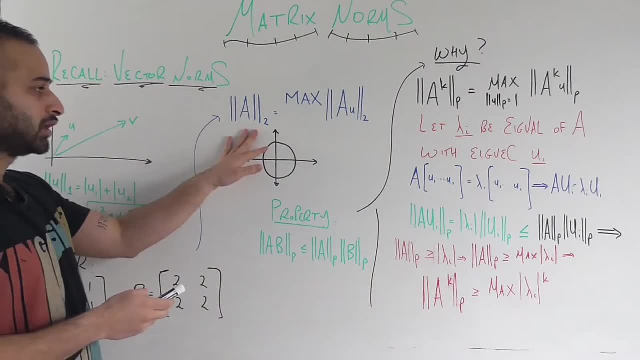 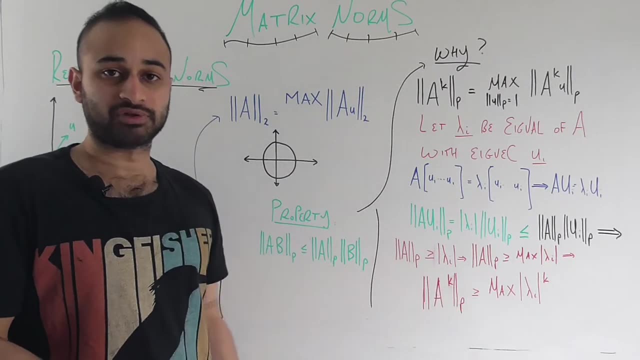 be concrete, we're taking the 2-norm of this matrix A. So the 2-norm of matrix A is given by the biggest L2 norm that this matrix is able to produce in terms of its output vector. So to say that more mathematically, if I do any vector u, 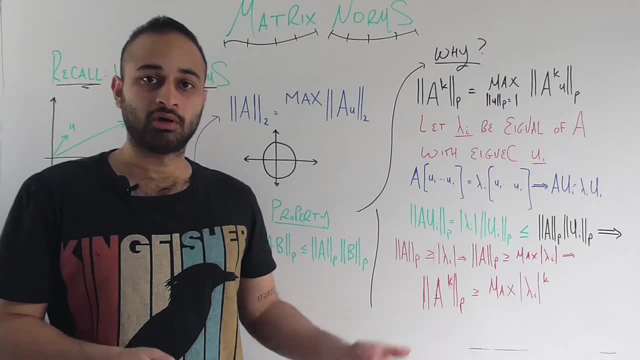 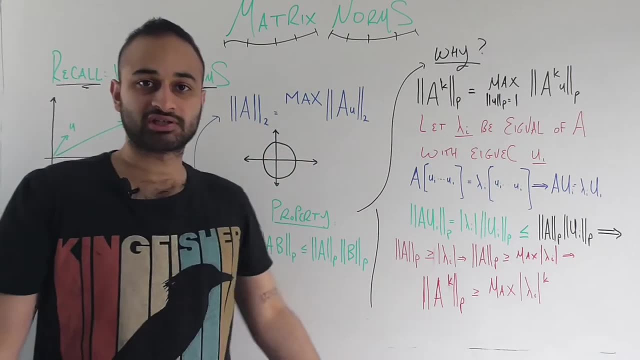 and I apply a. so I'm applying a to that vector u. what's the biggest that that output vector can get, And biggest is measured in terms of this two norm. I could switch these twos with ones, and now we're measuring it in terms of L1 norm. So that's really up to you and 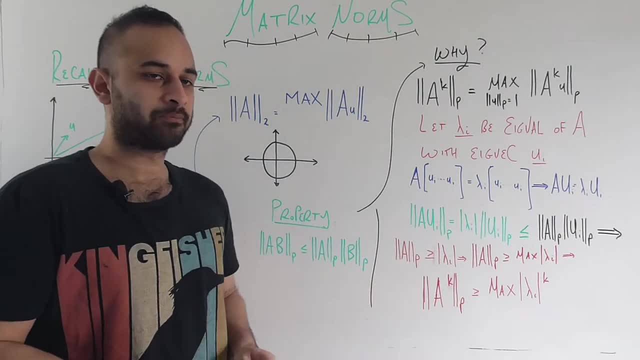 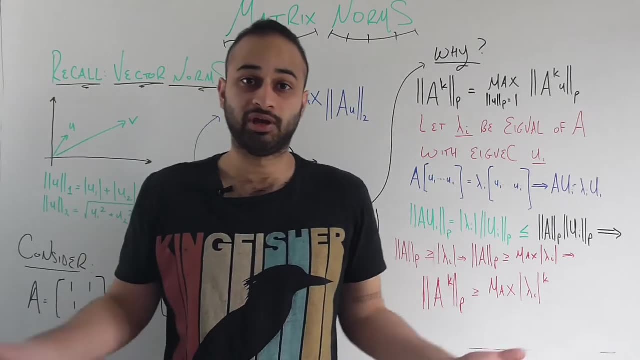 your application. There's one piece missing to the story, however. If I just wrote it like this, it's not a very good definition, because you can imagine that I can take this vector u and just make it arbitrarily big. I can just take it to infinity. 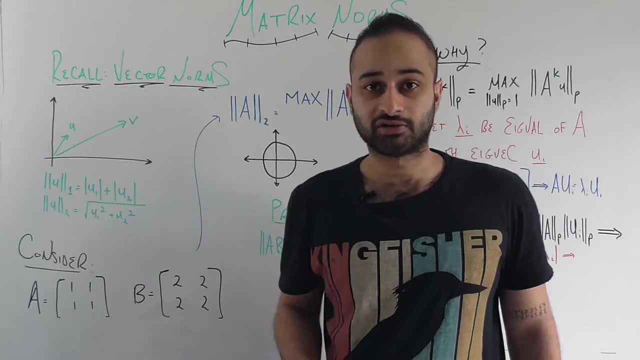 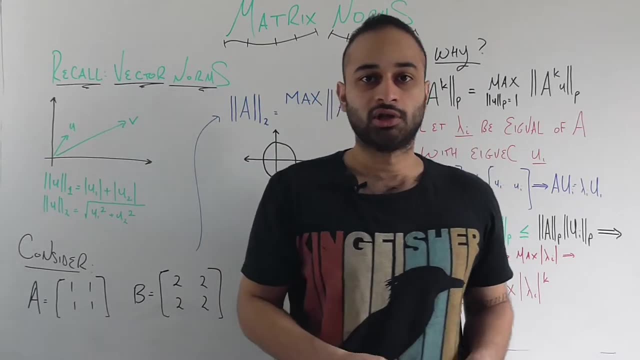 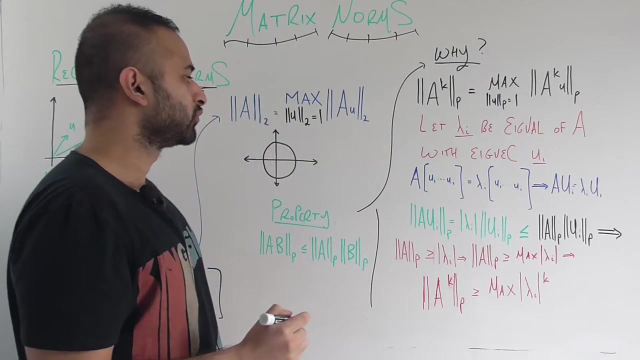 And if I put something infinite and apply it with either of these transformations, it doesn't really give me a good measure of which one is bigger. So we need to put some kind of constraint on the input. So we're going to say that the input u has to have L2 norm equal to one. A way. 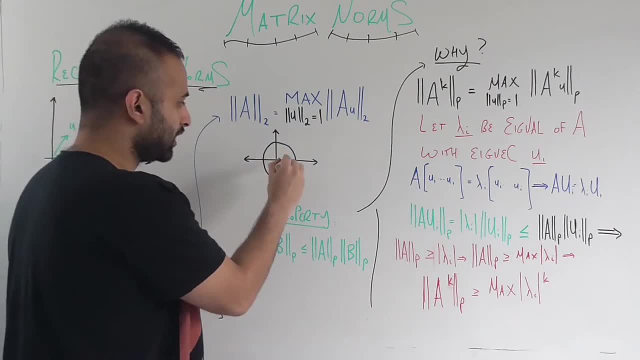 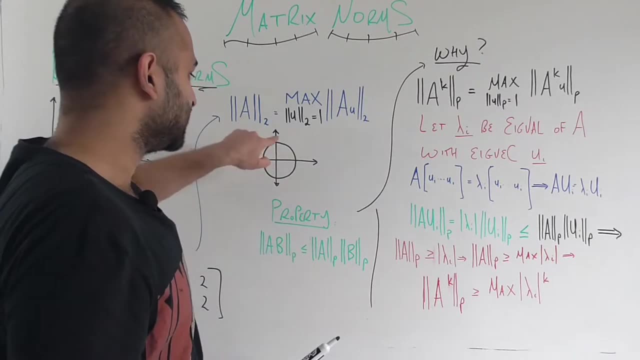 of saying that graphically is: this is the unit circle, so anything on this circle, any vector on that circle, is going to have L2 norm equal to 1, we're saying that: okay, matrix, you're allowed to take anything on this unit circle or in higher dimensions, a unit sphere or a. 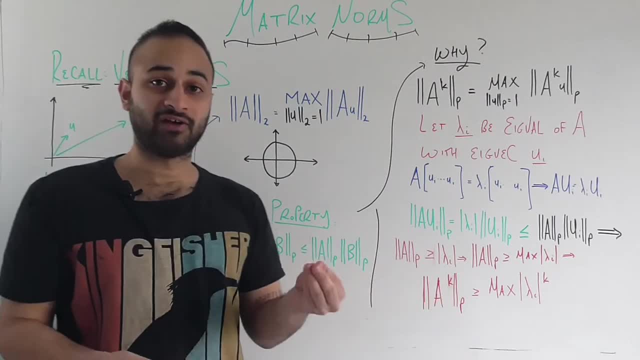 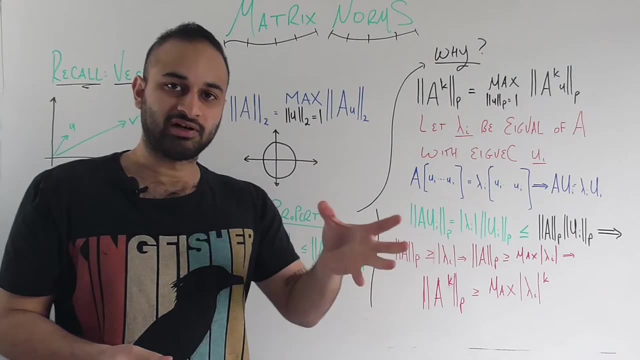 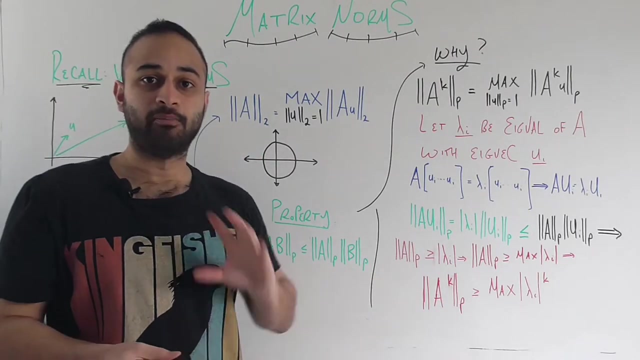 unit, hypersphere or whatever. you're allowed to take any vector on that circle and see how big you can get the output to be. So that way we're constraining the inputs. Every matrix is able to only choose from these inputs and we're gonna say that the L2 norm of that matrix is given by how big the 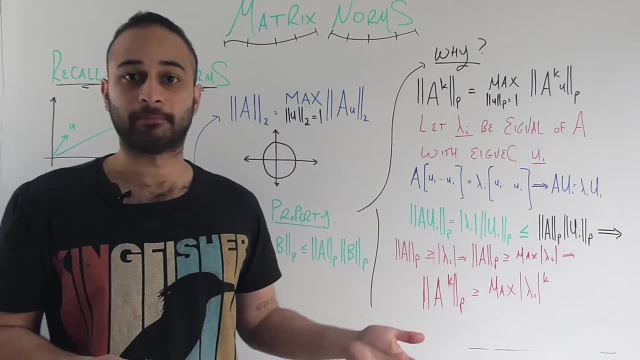 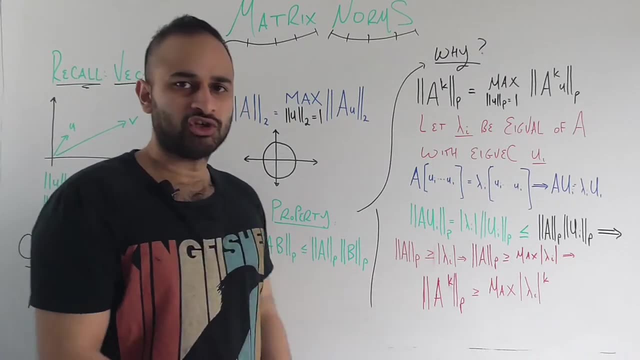 output can be, given that the input has to lie on that circle or sphere. Okay, So that's what it means to take the norm of a matrix. Now, this video wouldn't be complete without giving you an application of why this is useful, As you. 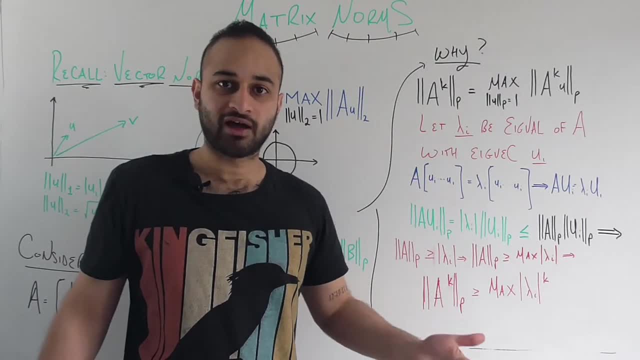 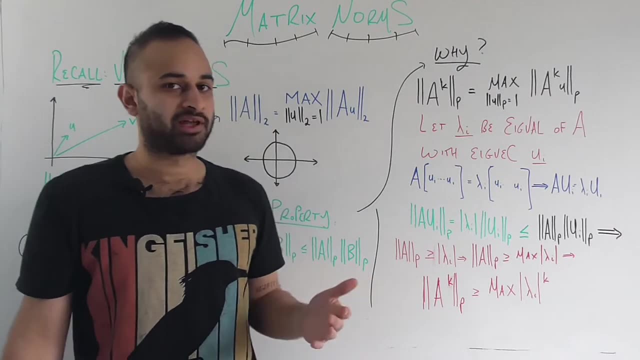 know, on this channel, I don't really like to talk about math for the sake of math. I like to talk about math because it's useful for some kind of data analysis or some kind of application. So let's look at a quick application of why this. 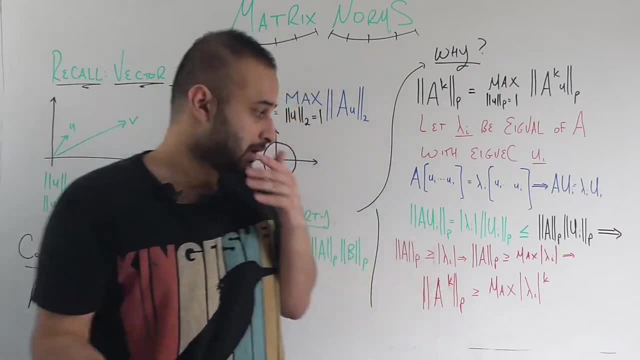 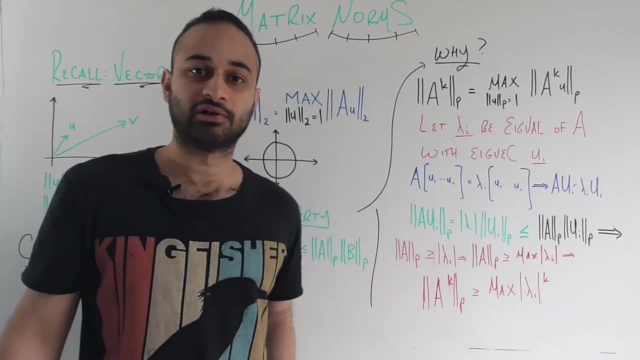 notion of a matrix norm is actually useful. So quickly a property about matrix norms. that I won't prove, but if you really are interested, please leave a comment and I'll give you a link to a good detailed description. But this basically says that A times B. 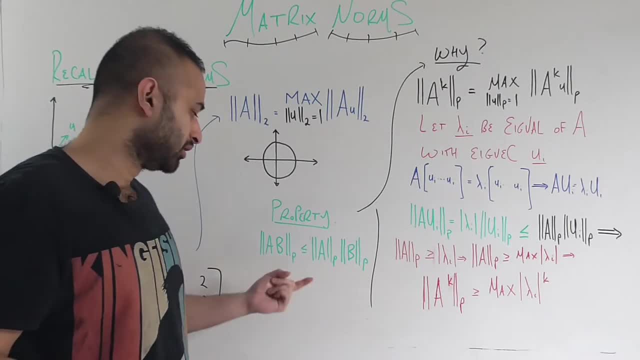 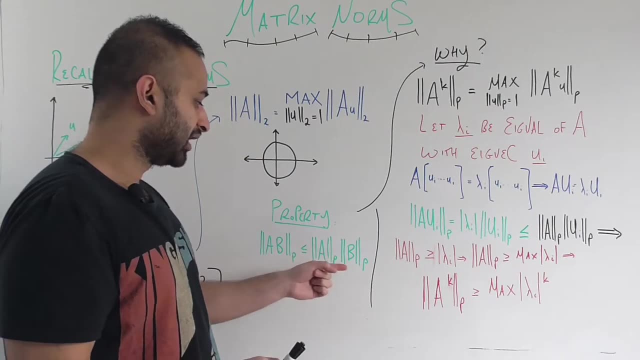 so if I take the product of two matrices and I ask for the p-norm of that, it's going to be less than or equal to the individual p-norms. So p-norm of A and p-norm of B multiplied together. 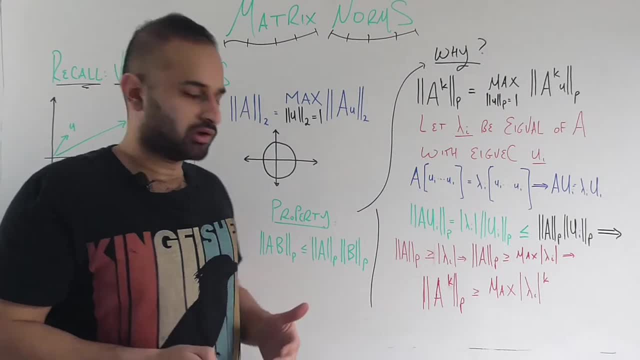 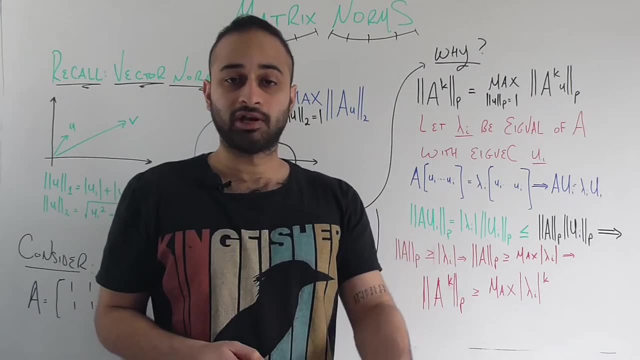 So this is kind of in the spirit of a triangle inequality, but you can think of it however you want to think of it. Now, using this property, we're going to be putting a bound on a very special matrix form, namely a matrix power. 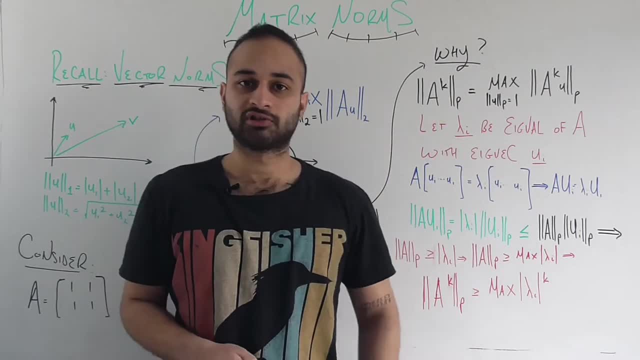 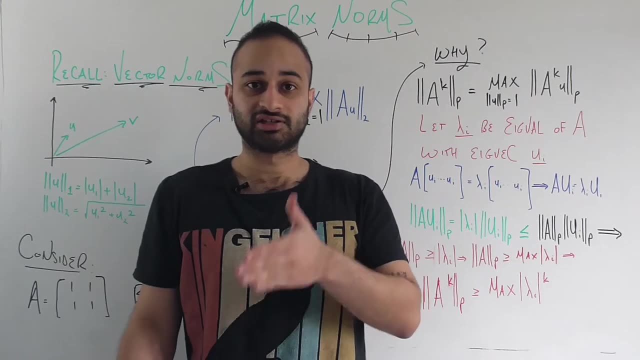 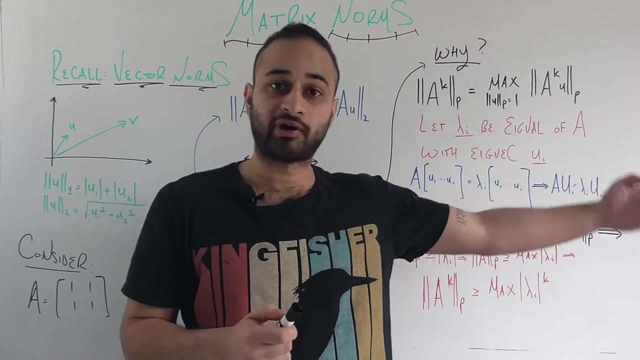 A matrix power is when you take a single matrix and raise it to the power of some number, k. This form is very important in data science because, if we think about what a matrix is again, it's a linear transformation And usually in data science or machine learning we're doing some kind of algorithm where we apply this transformation over and over and over again. 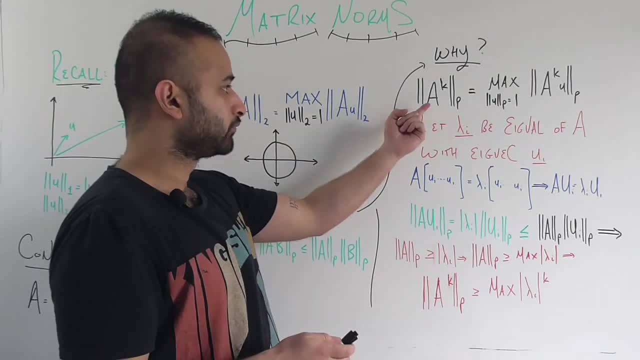 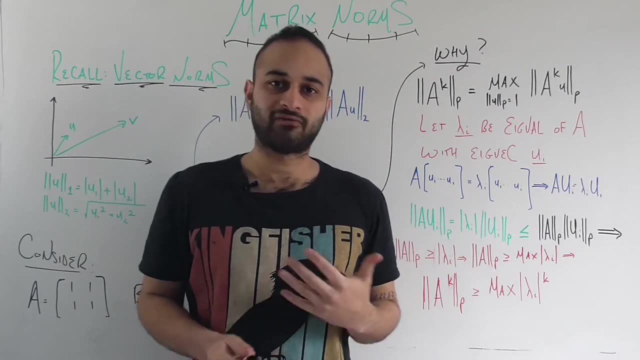 And that kind of ends up being equivalent to taking a matrix power. So we want to figure out: is there a bound on this matrix power? Can we lower bound it in some way? The reason we want to find a decent lower bound is because there's always a chance. 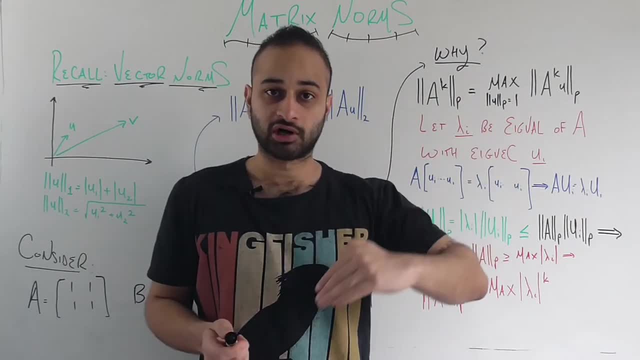 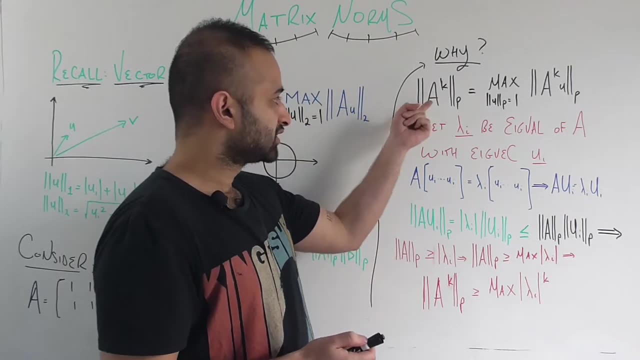 that, as we take successively higher powers, this thing is going to go to zero, which could cause problems for our machine learning algorithm. So we want to see if that's happening or maybe not happening. So this, just based on the definition that's written right here, is going to be equal to this. 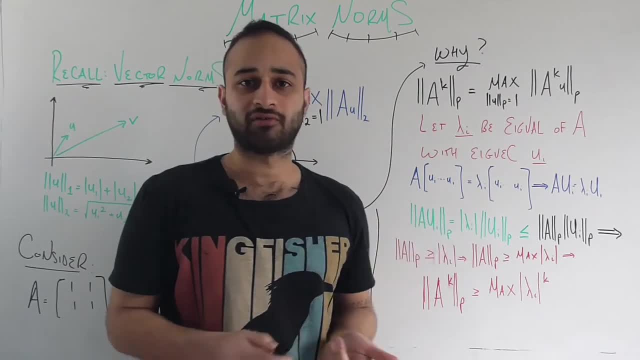 But just based on that definition, it doesn't seem too easy trying to find a good bound. So let's go off of that. So let's go off of that. So let's go off of that. So let's go off of a couple of other things we know. 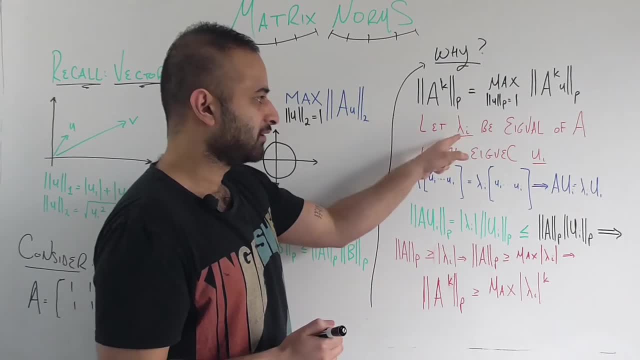 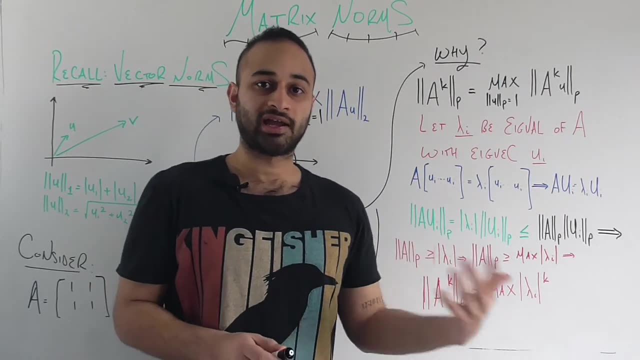 One thing we're going to say right off the bat is that let's let lambda i be an eigenvalue of a with corresponding eigenvector u sub i. So, going back to our discussion on eigenvalues and eigenvectors, this is just saying that a times ui is lambda i times ui. 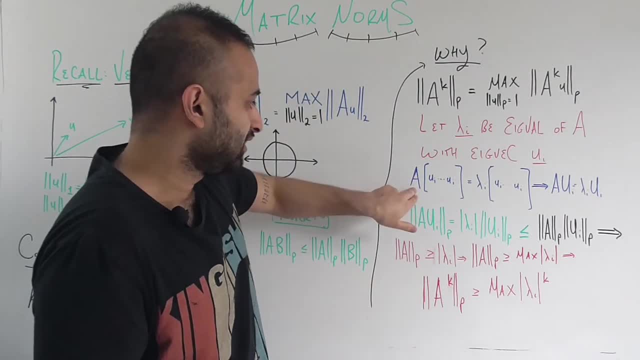 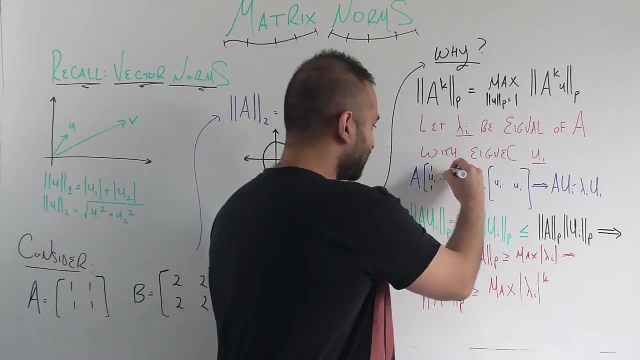 Definition of an eigenvector. That means that a times a matrix full of these ui's. So to be explicit here, the first column is ui, The second column is ui. All the way to the last column is going to be ui. 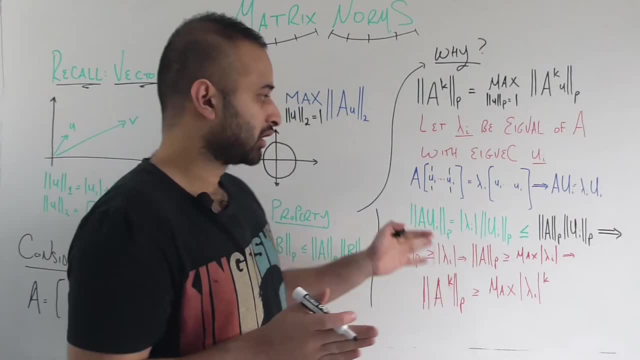 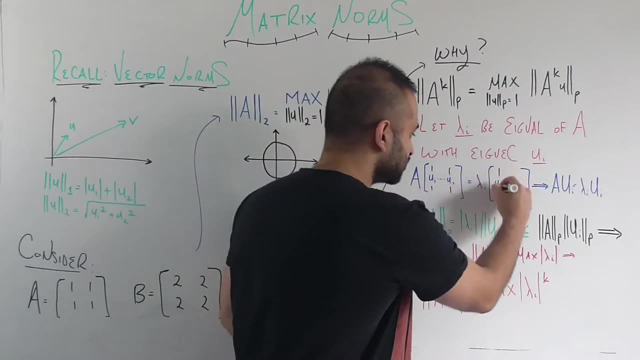 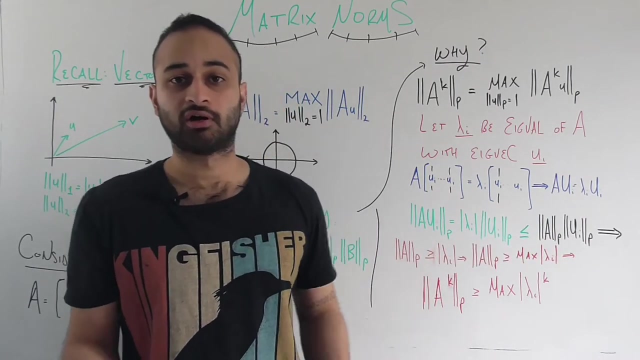 So this is a matrix full of ui's. We're going to call that matrix big ui. This, of course, is equal to lambda i times ui, lambda i times ui, all the way to lambda i times ui. Again, based on the definition of what it is to be an eigenvector and an eigenvalue. 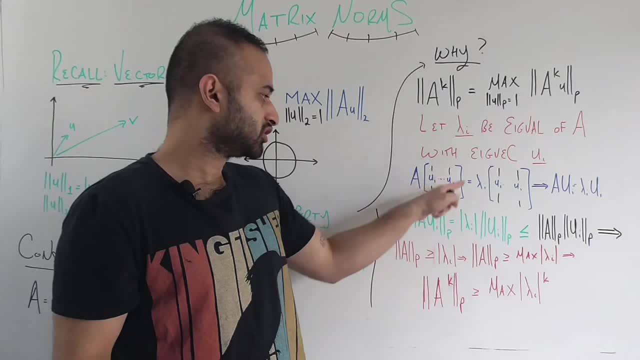 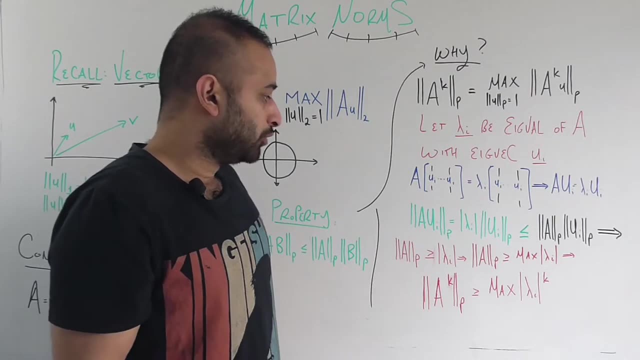 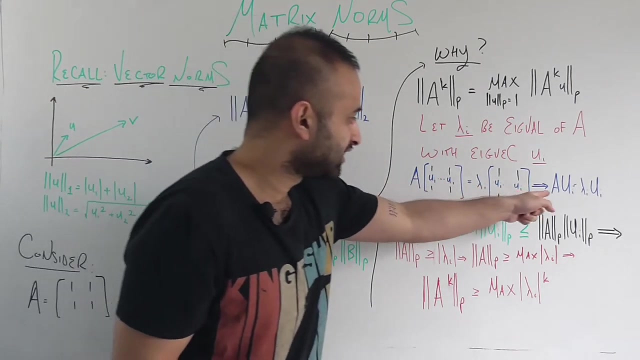 So in matrix notation we can say: a times ui is equal to lambda i times ui. Nothing too fancy Going on here. Now we can use this property here to go ahead and find our bound, So we can put this left hand side. 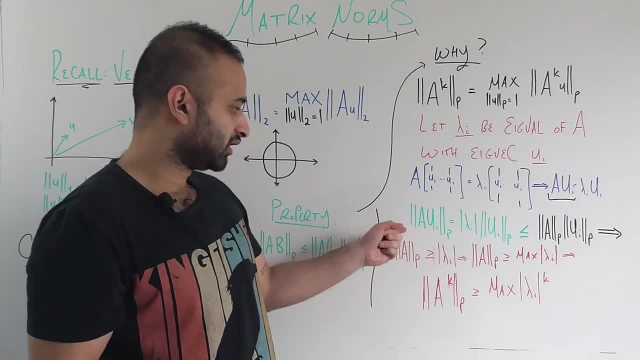 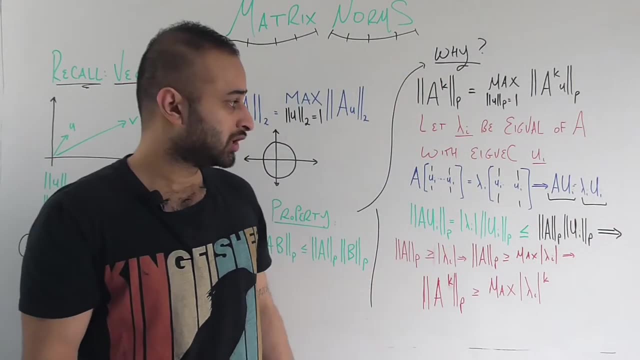 So this a times ui in our p norm. That's what I've done here. That, of course, is equal to taking the p norm of the right hand side because, as we've seen, they are equivalent. This lambda i, being a constant, can just come out in absolute value. 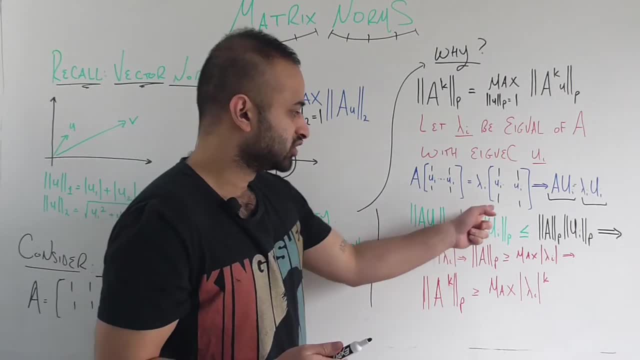 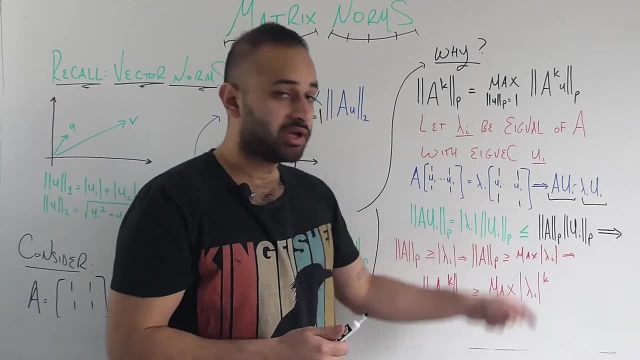 So that's why we have absolute value of lambda i here, Leaving just ui p norm Right there. All right Now. this is less than or equal to the individual p norms multiplied together. Why, Based on this property we just looked at here, 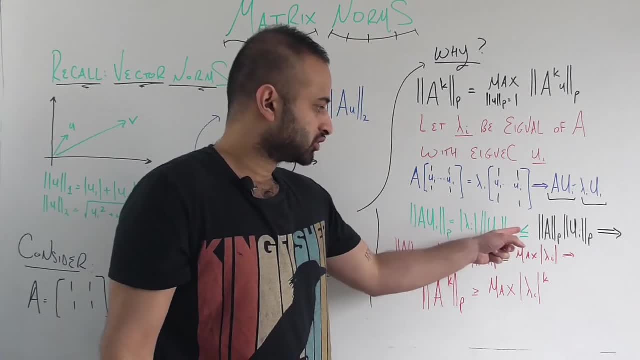 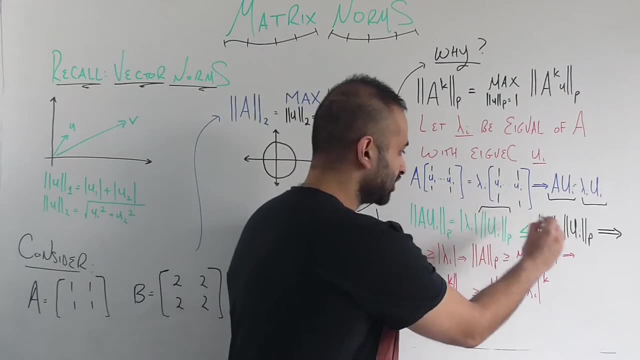 So that means that this quantity here is less than or equal to the p norm of a by itself times the p norm of ui by itself. Now we see a ui p norm showing up here and a ui p norm showing up here, So we're going to cancel them out, leaving just that lambda i in absolute value. 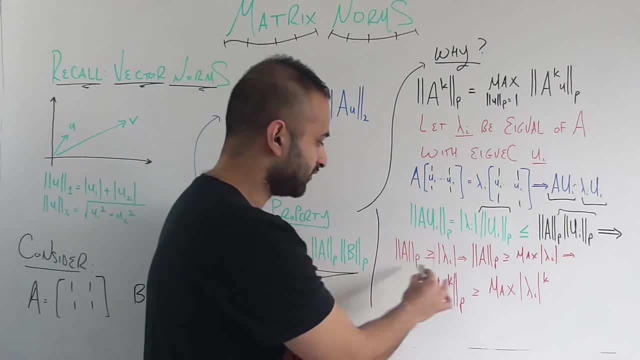 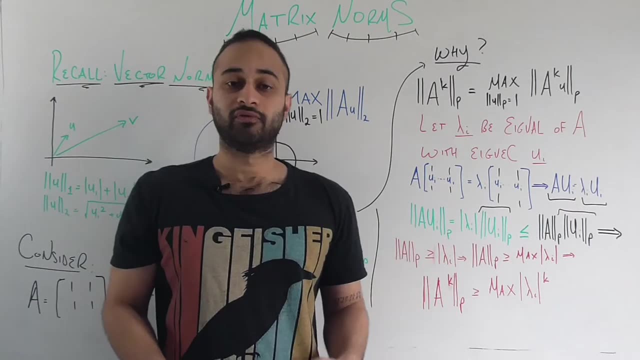 Is less than or equal to. So I guess I've written the opposite way. here We see that p norm of a is greater than or equal to absolute value of lambda i. So if you need to pause for a second, think about all the steps, write them down, go ahead. 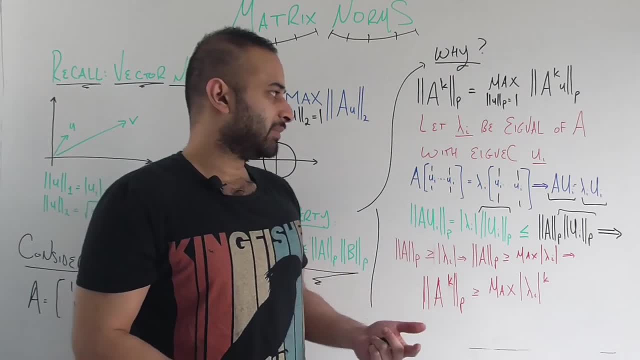 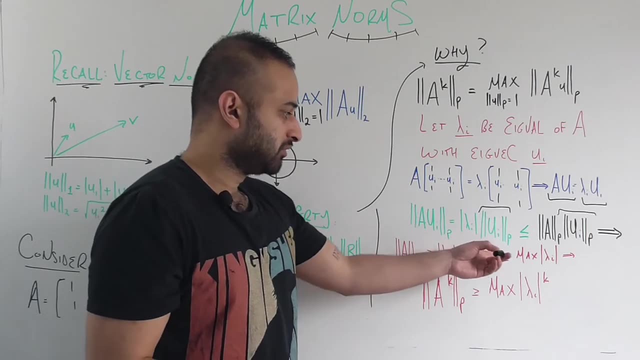 But just to move forward here- notice that I didn't say anything about lambda i, which eigenvalue it is So arbitrarily- I can say that that means that the p norm of a has to be bigger than or equal to the largest eigenvalue of a in absolute value. 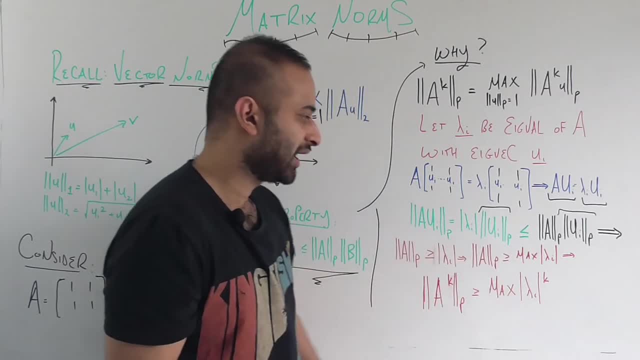 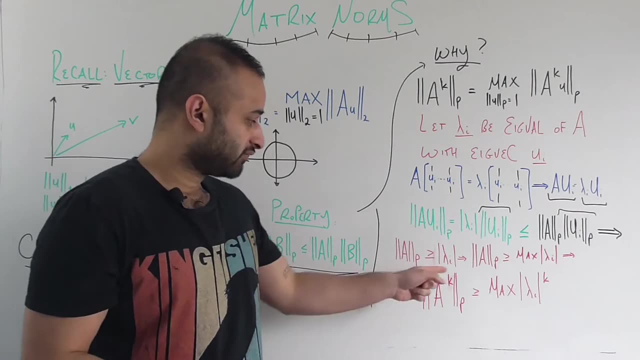 Okay, So that's what I mean by max lambda. i right here. And to complete the story, because, remember, we're trying to tell some story about the matrix power, that would mean that a to the power of k, its p norm is greater than or equal to the maximum eigenvalue in absolute value, also to the power of k. 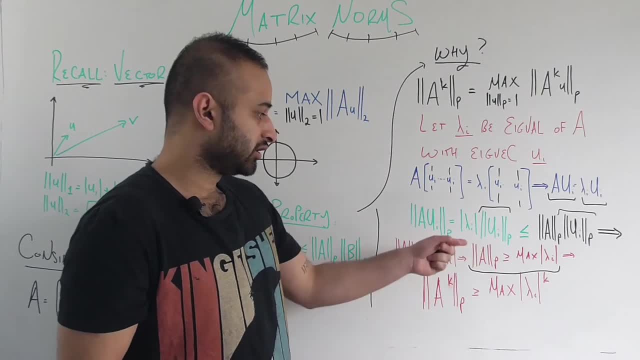 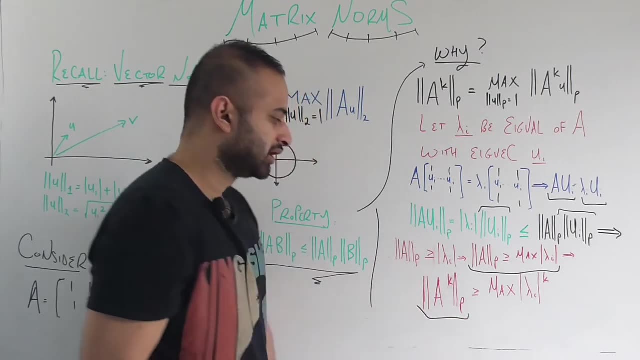 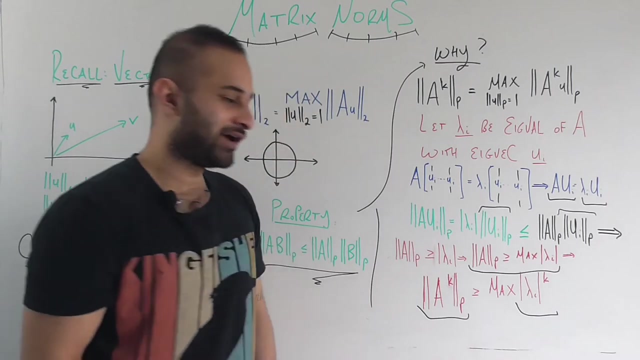 So what I've done there is just take this inequality here and just iterate k times and I get this inequality here. Now, why is this useful? Why is it useful to know that the p norm of a to the power of k is going to always be bigger than or equal to this quantity? max lambda i, absolute value to the power of k.